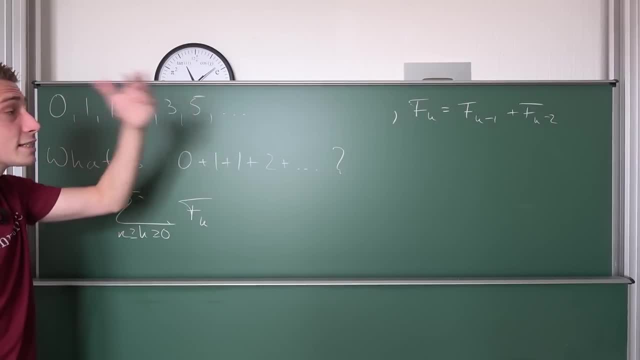 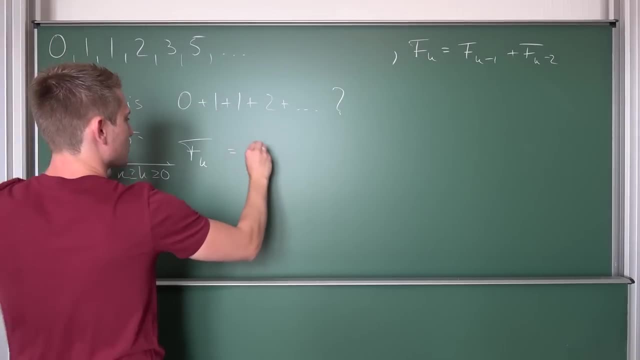 Okay, So just as a little side note here, This is how they are defined. And now, just for trying out purposes, Let us plug the Fk into here and see what we are going to get. We are going to get the sum being bounded between 0 and n. 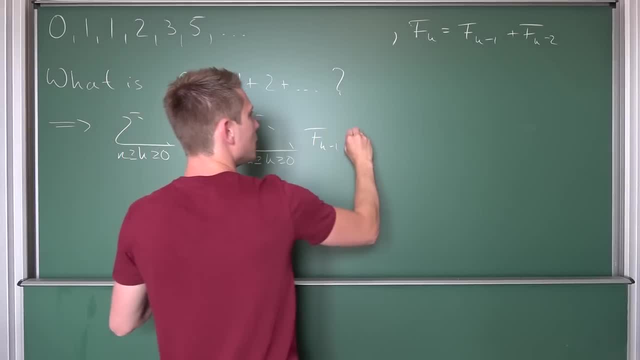 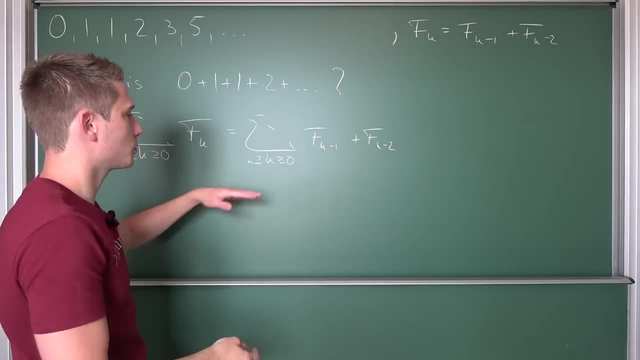 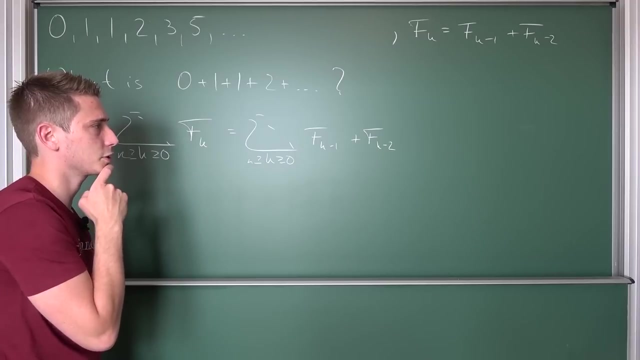 Of Fk minus 1 plus Fk minus 2.. Okay, What would happen if we were to plug in our indices Right here? Okay, With 0, we are going to get negative 1 Fibonacci number plus the negative 2 Fibonacci number. 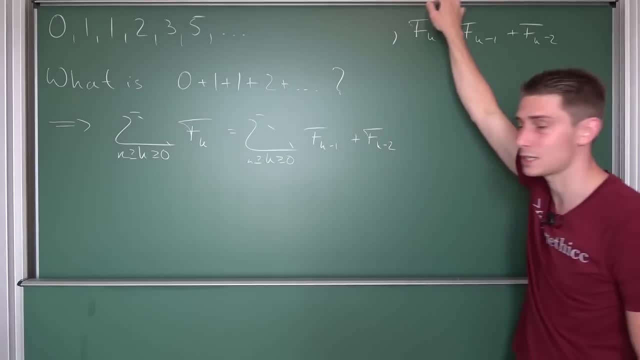 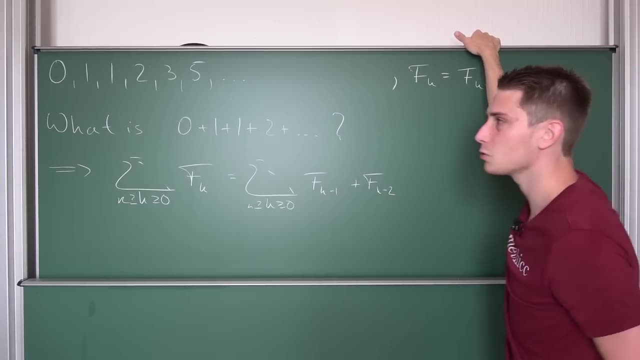 Doesn't make any sense, Right? I mean, it does make perfect sense. You can extend the Fibonacci numbers to all the real numbers- I did do so before- But we are strictly going to speak about the pulse of Fibonacci numbers. So Fibonacci numbers of the negative order really don't make any sense right now. 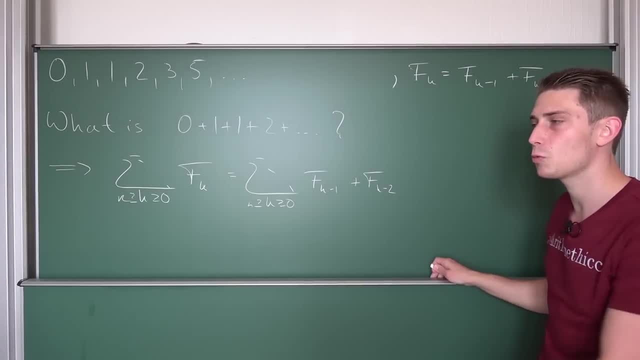 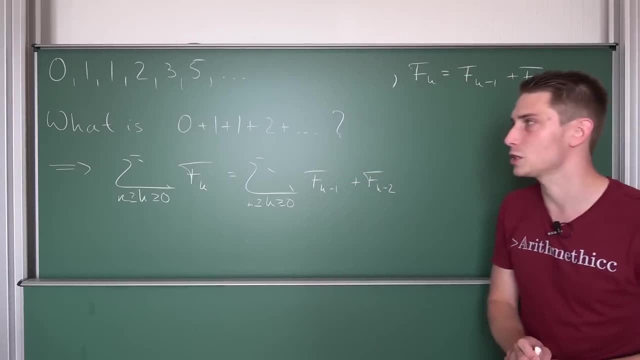 This is why we need to get a bit creative Working around with the indices And we are going to do a little index shift here on our original recursive definition. And this index shift actually does make perfect sense If you start summing up the first few Fibonacci numbers and try to see a pattern here. 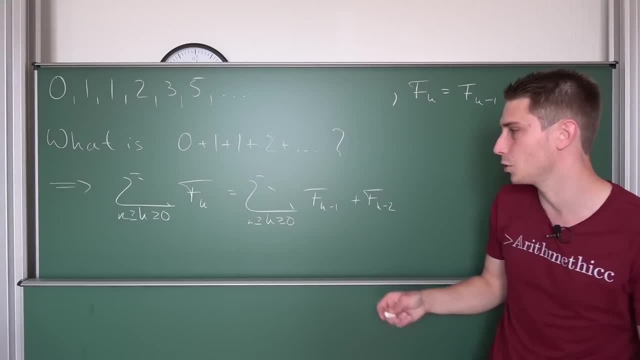 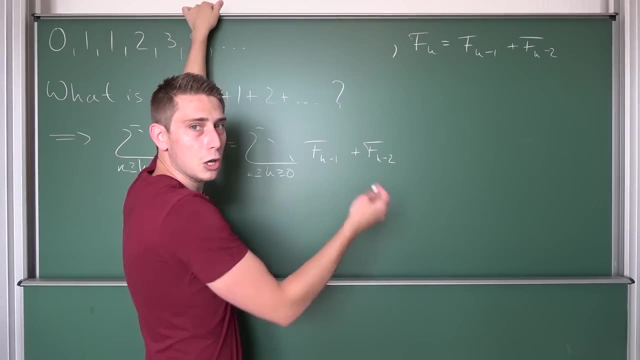 This is what we are going to do at the end, to motivate it a bit further. So what we are going to do is we are going to get rid of those negative indices. Our lowest negative indices would start at negative 2.. So why not add negative 2.? 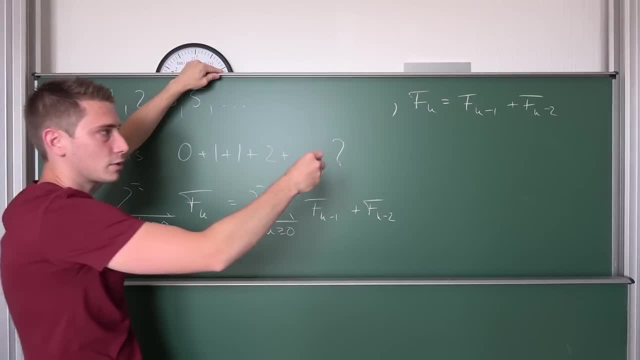 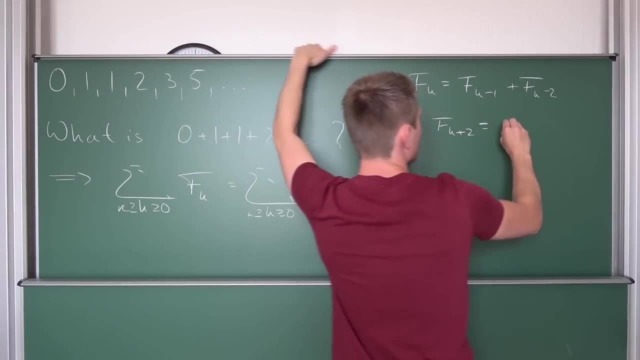 But add a 2 to each and every index. Okay, It does make kind of sense. We are going to do an index shift from k to k plus 2. Meaning Fk plus 2 is just equal to Fk plus 1 plus Fk. 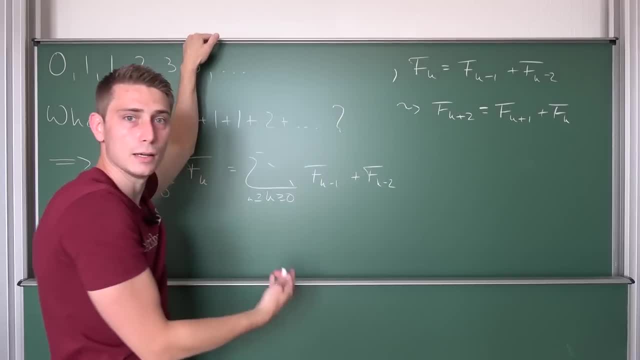 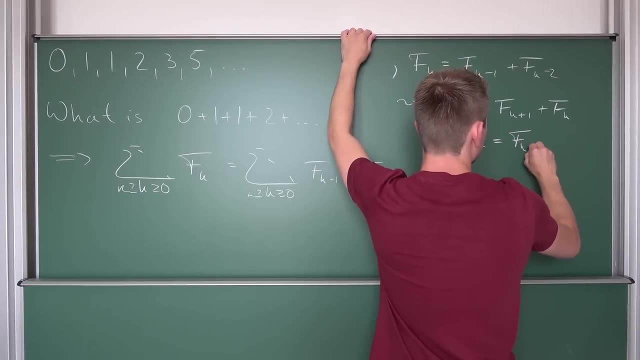 Hey, There we go. This got us rid of this weird problem with the indices Meaning we are going to solve for Fk. Fk does nothing but Fk plus 2 minus Fk plus 1.. Now we can plug this into here. 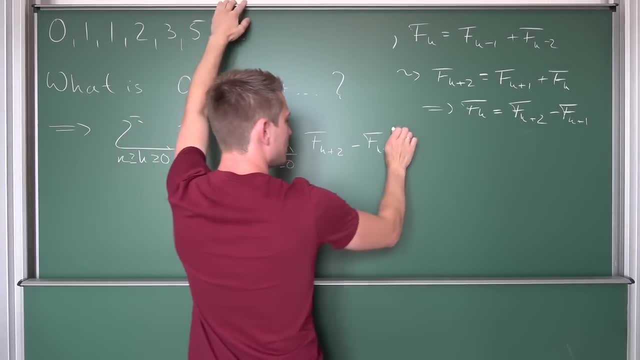 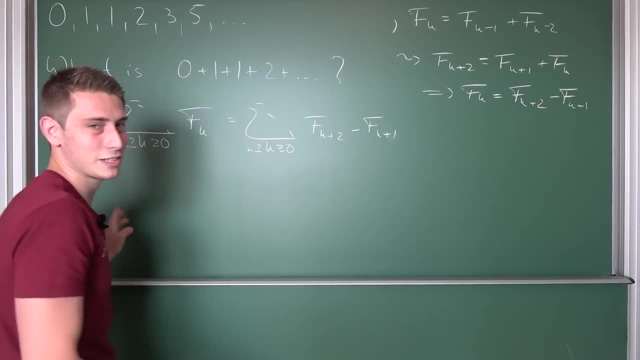 So this is Fk plus 2 minus Fk plus 1.. And this already got rid of the biggest problem here. Now we can start computing and see if we can find a certain nice pattern. Oh yeah, We are going to do so. 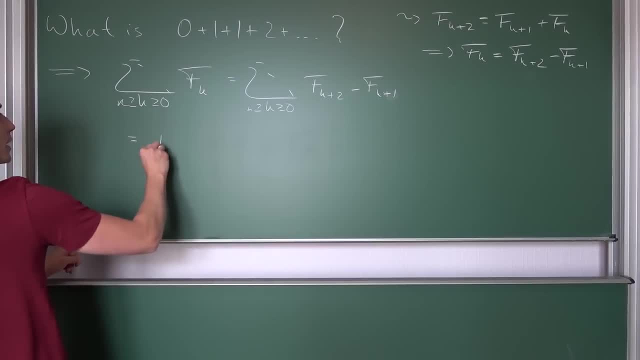 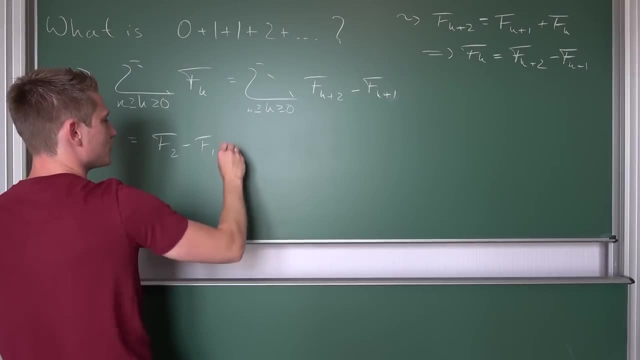 We are going to do so, mate, Let's plug it in with 0.. We are going to get, Okay, Plugging 0 into here. This is F2 minus F1.. Okay, Next up, Plugging 1 into here. 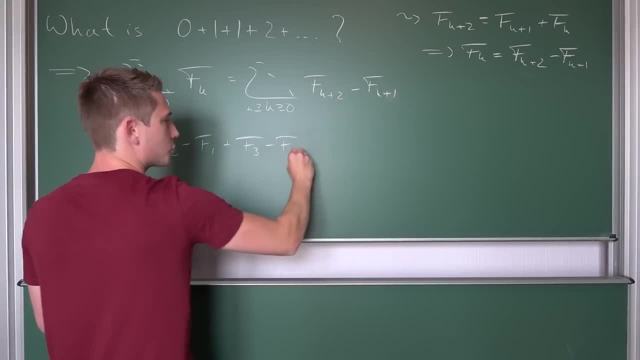 This is going to give us plus F3.. Minus F2.. Mmm, That's spicy mate. Are they going to cancel it? Yeah, They are going to cancel it. Additive inverse is my boy. Now we are going to add: 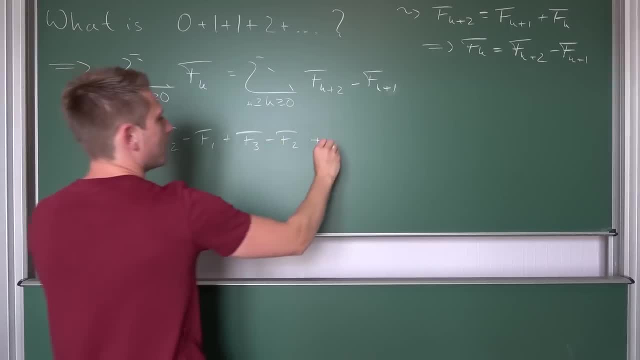 Let's go through a few more iterations: F4 to it and subtract F3 from it. Pretty easy pattern. Then we are going to go ahead and sum a bunch of stuff up. Then for the n minus 1 iteration, we are going to get Fn plus 1.. 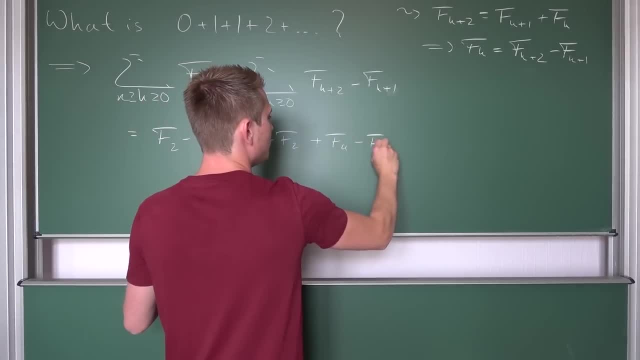 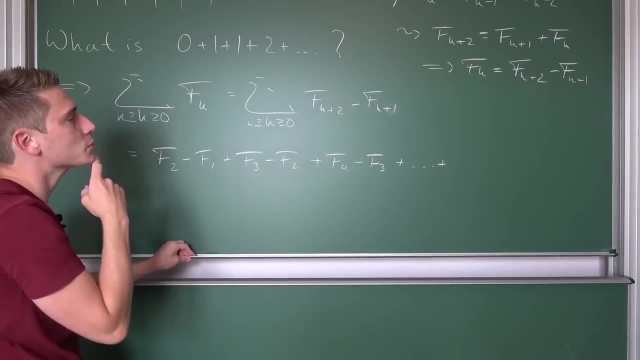 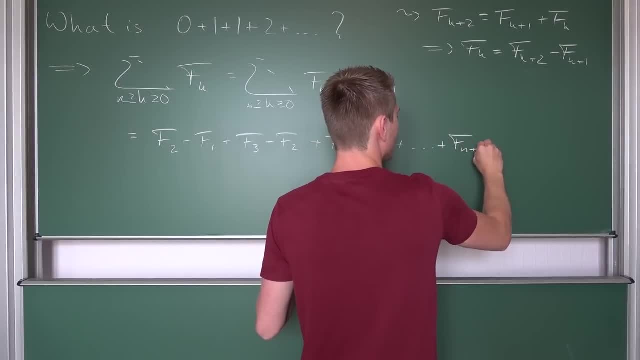 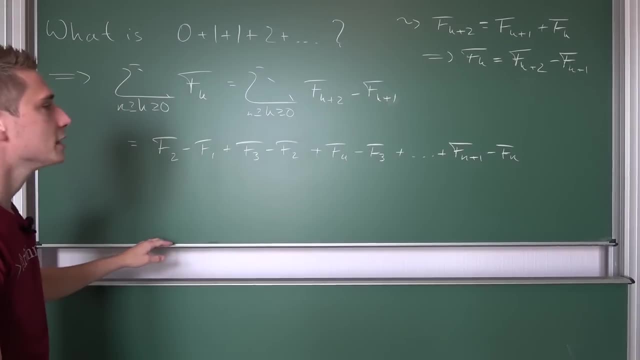 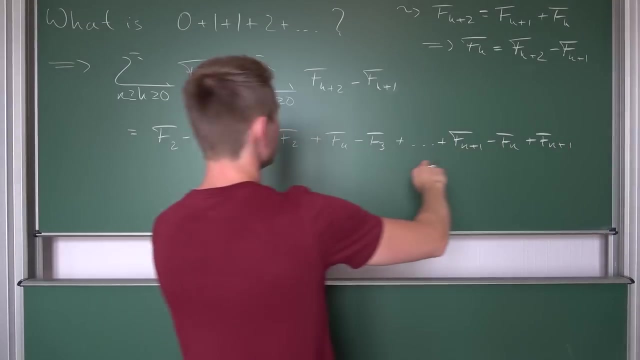 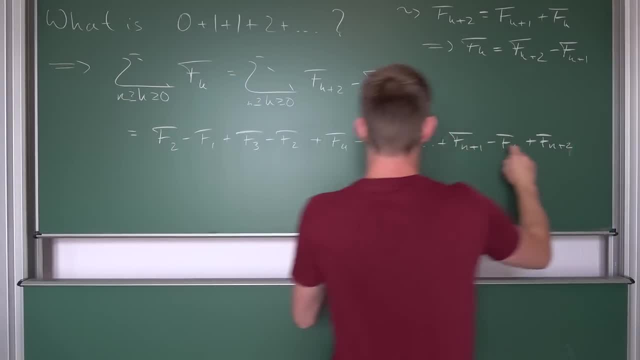 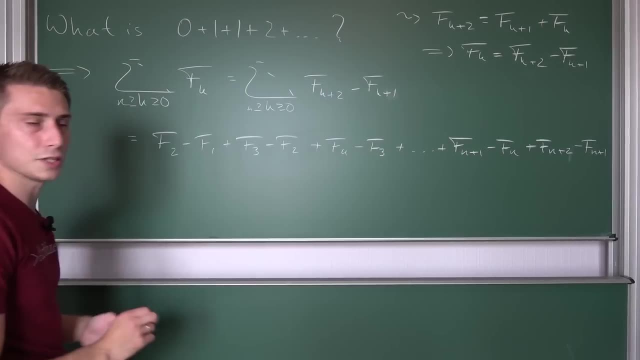 Fn plus 2.. I'm terribly sorry. Yes, Fn plus 2.. Minus Fn plus 1.. And now you can see that a lot of stuff is going to cancel out. It's a well, it's a telescoping sum that we 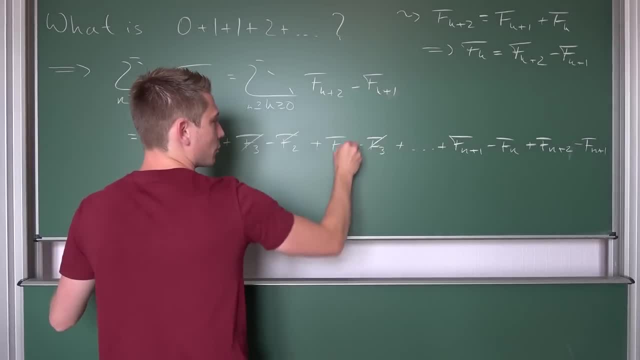 are having here f2 and f2 is going to cancel out f3 and f3 is going to cancel out f4 and f4 is going to cancel out. Also, fn plus 1 and fn plus 1 are going to cancel out, Obviously. 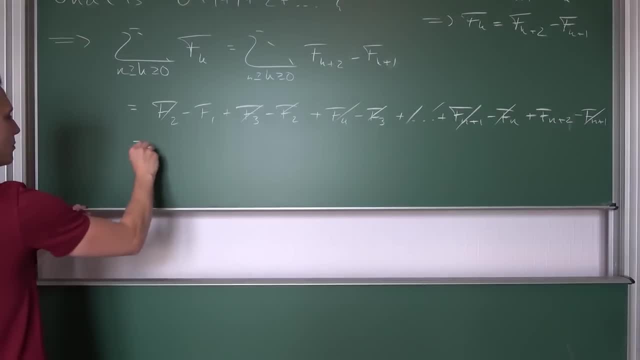 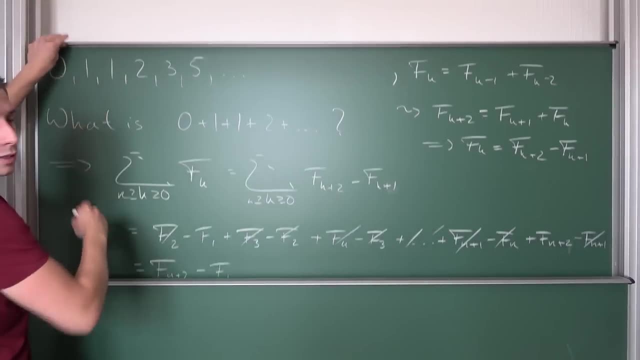 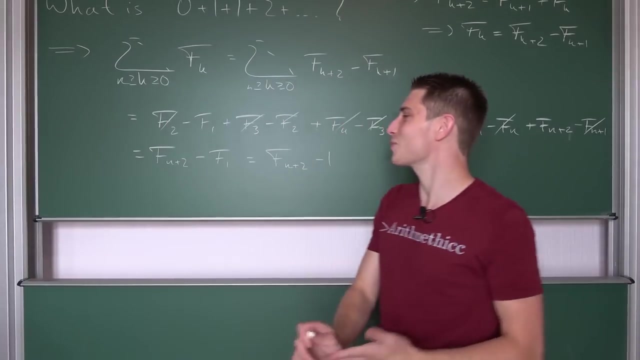 fn and fn are going to cancel out, leaving us with simply fn plus 2 minus f1, and f1 is exactly the first Fibonacci number, which is 1.. fn plus 2 minus 1.. It was really easy, right. I mean this is pretty cool. We are going to be left with just this expression, which is: 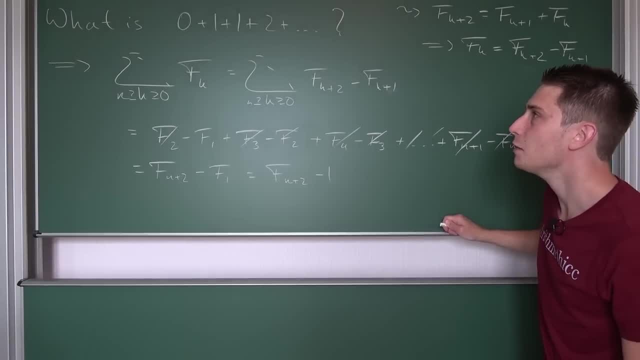 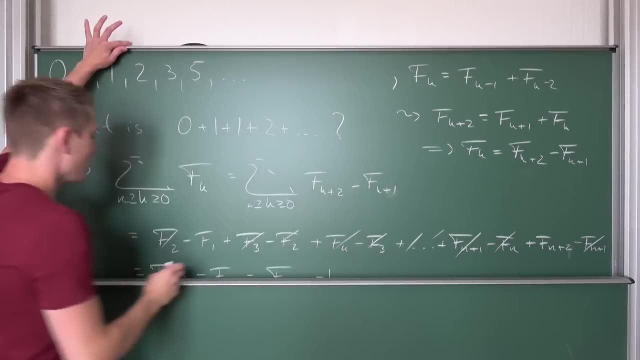 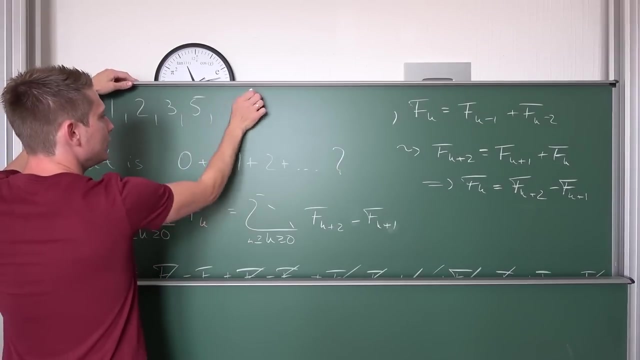 pretty cool. if you ask me, It's pretty easy to evaluate Meaning if we were to sum up to the, let's say, 6 Fibonacci numbers. So 6 Fibonacci number is 5, then we are going to get ok. So our n was 6, meaning we are going to get up to 8 in our index. So the next one. 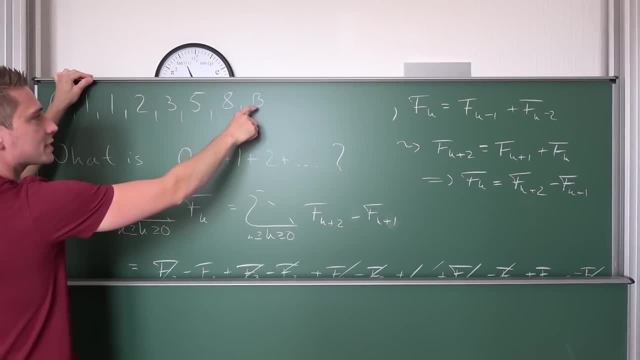 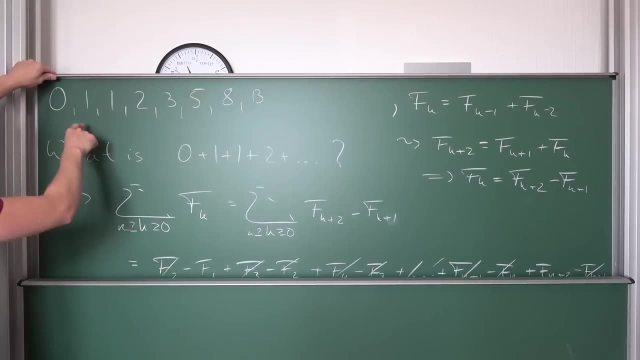 is going to be 8 and after that we are going to get 13.. Meaning this makes 13 minus 1 is 12.. Ok, As our answer- Let us see if this works- So we are going to have 1 plus 1 plus 2 is. 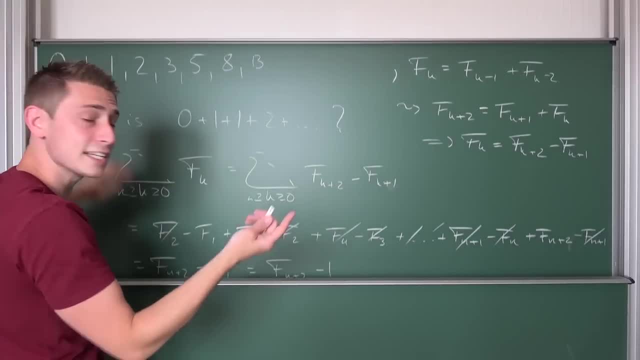 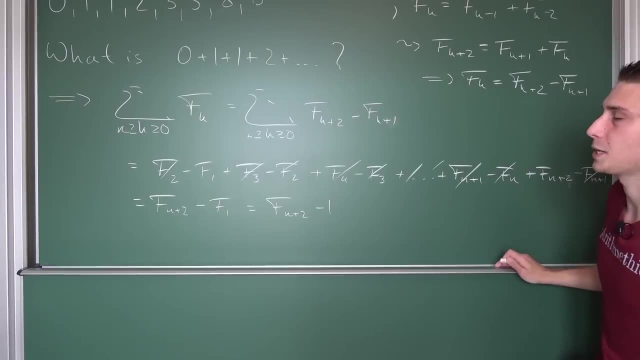 going to give us 4 plus 3 is 7 plus 5 is going to give us 12.. That's worked out pretty nice, right? And we can already see this pattern if we just start to compute a bunch of stuff. So let us compute the first few Fibonacci numbers. Sums are, let's say, 0 plus 1 plus. 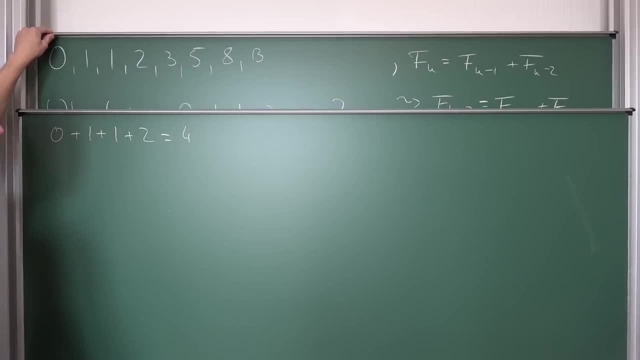 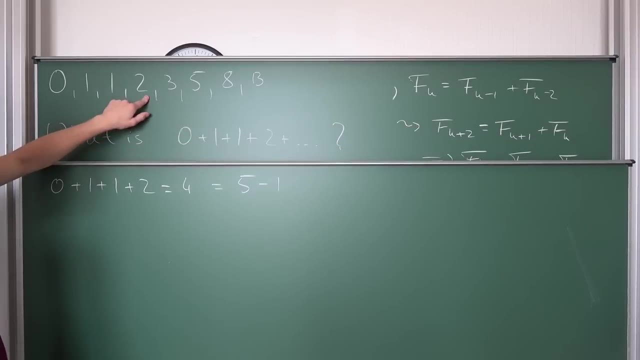 1 plus 2.. It's nothing, but obviously 4.. And what is 4?? Well, 4 is nothing but 5 minus 1.. Ok, Meaning we start here at this Fibonacci number, then we are going to add two more indices. 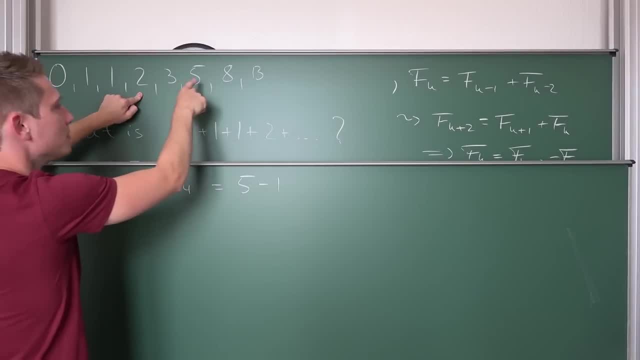 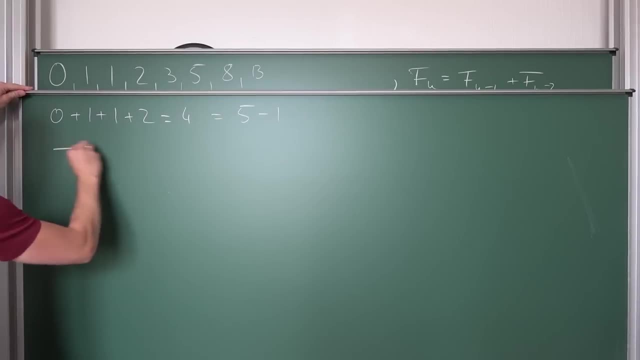 to it. So we are going to go up to the. this was the fourth Fibonacci number, that is, the 6. So F6, which does make sense with our formula that we got, and then subtract 1 from it. What about the next one? 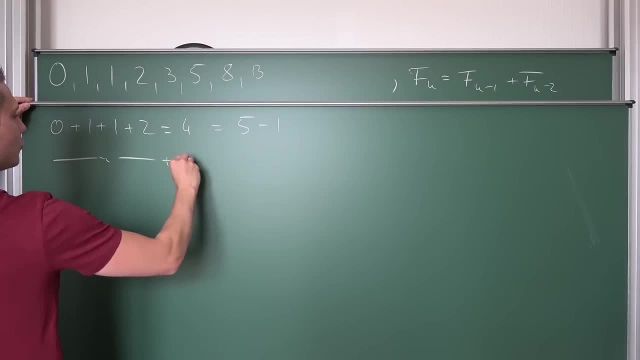 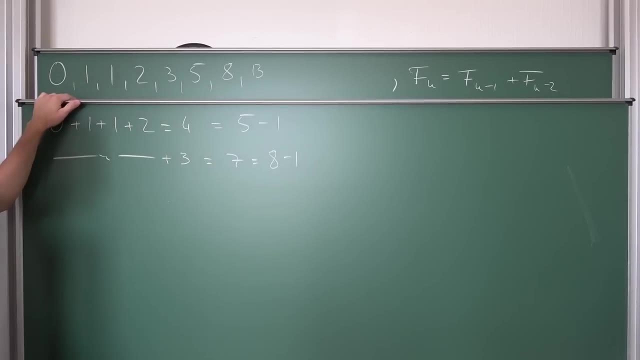 Let us do this, and then we are going to add the 3 to it. Ok, That's obviously going to give us 7, and 7 is 8 minus 1.. Okay, and this does make sense, from 3 to 8. 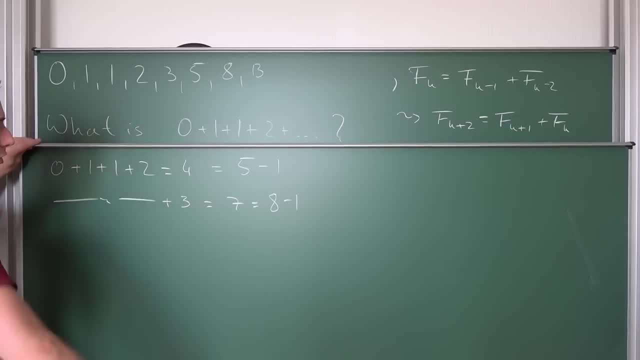 Two more Fibonacci numbers and then subtract 1 and he can just continue this process. if you were to add a 5 to it, We're going to get 12.. We just hit this case and then we're basically done. I hope you enjoyed this video. 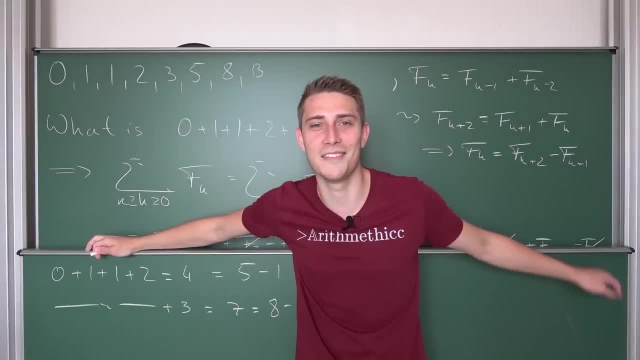 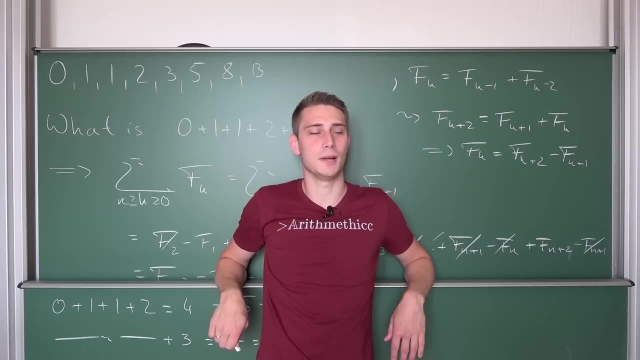 Please like, subscribe and comment. share and leave a like. If you want to support the channel a bit more, buy us t-shirts. aid creators. support the channel on patreon. I'm so mentally disabled at this point I'm gonna take this video and wish you guys a flamboyant day. Ciao.